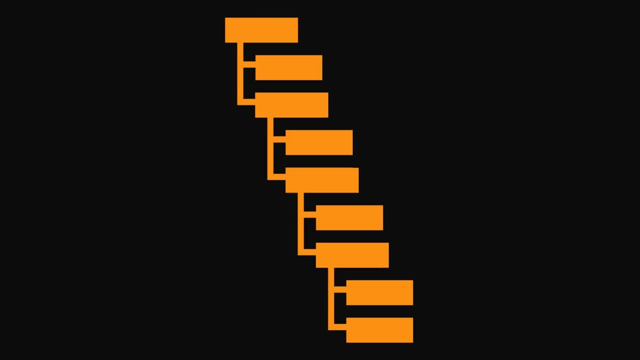 structure. often things can get very complicated and long lines and long branches can branch out from your file folder structure And I'm sure you've had the experience at getting to the bottom of one of those long lines and then being frustrated discovering that the file or the 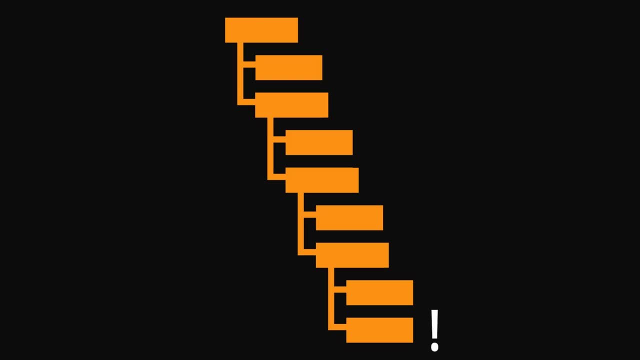 document or the picture you were looking for does not reside there at all, And then you have to back up and go looking elsewhere. Where would I have put this particular file? Well, today I want to show you a simple but very powerful way to structure all of your files. 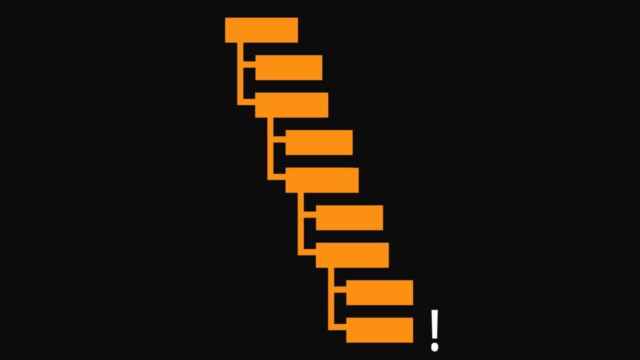 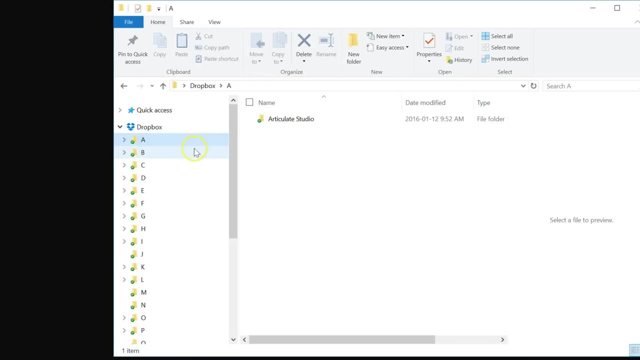 In what I call the ABC Folder Method. What exactly is the ABC Folder Method? Well, let me jump to my folder structure right here, And we're actually looking at my actual Dropbox folder. So you will notice, at the top level I have 26 file folders, All of them listed A through Z. I've got the entire. 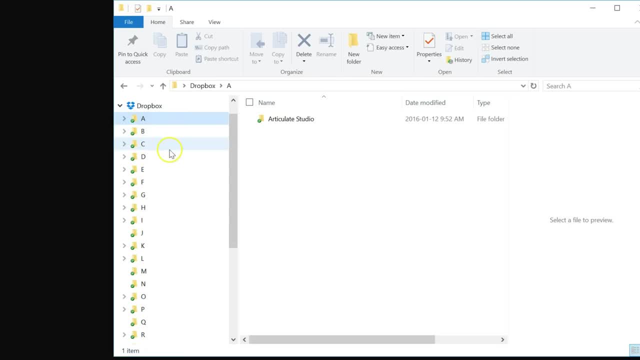 alphabet here in front of me. The way that the ABC file folder structure works is that we want to be able to quickly get to the files that we are after and not have to expand and collapse multiple file folders to get to the thing that we're looking for. 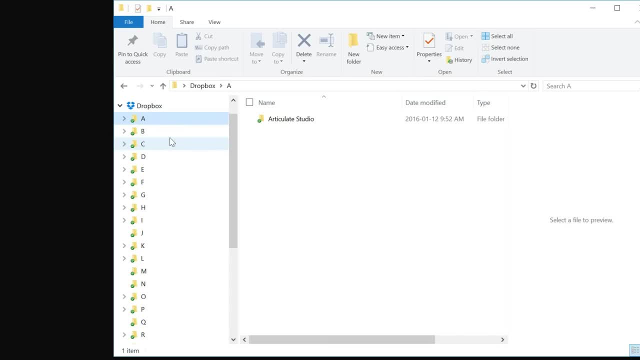 In fact, we only want to click twice to get to the file that we're looking for. So the reason that we start with the alphabet is that we want to group our subfolder beneath the based on the letter in that alphabet. So let me expand my C folder to give you an example. 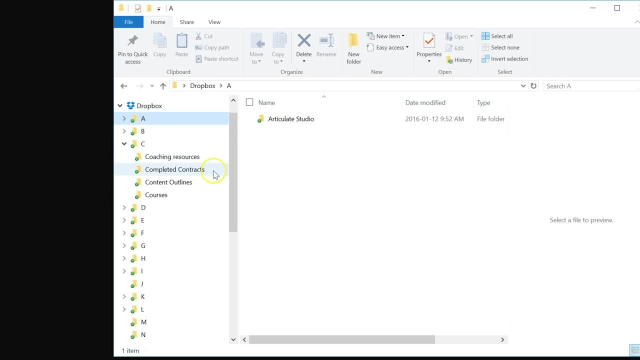 Within my C folder I have coaching resources, completed contracts, content outlines and courses. These really are not related to one another in any way, except for the fact that they all begin with C, So if I'm looking for information about courses, 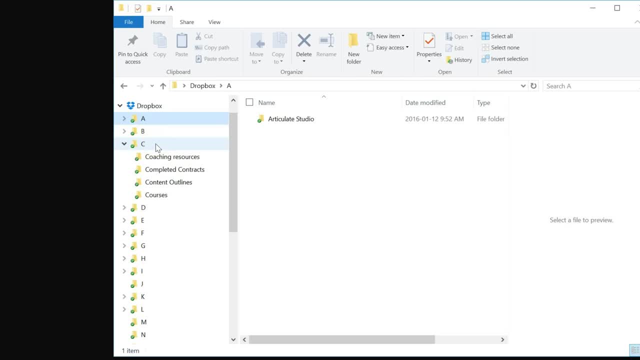 I know it's going to be under my C folder. I don't have to look anywhere else And when I click on my C folder I have my files right there. So only two clicks. I can click on the C and then the courses. 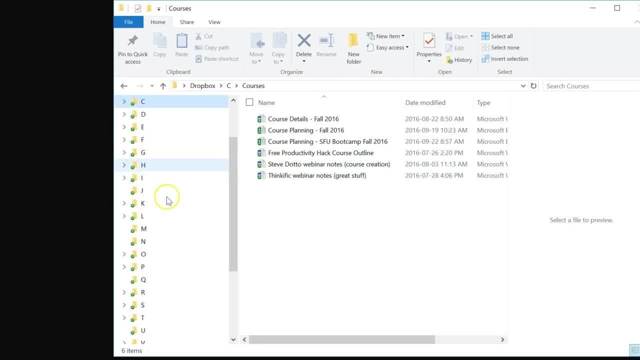 and then directly to the file that I'm looking for. Let's take a look at another example. Let's expand my P folder. Here we have payment pictures, pricing products and public speaking training- Again not really related to one another.